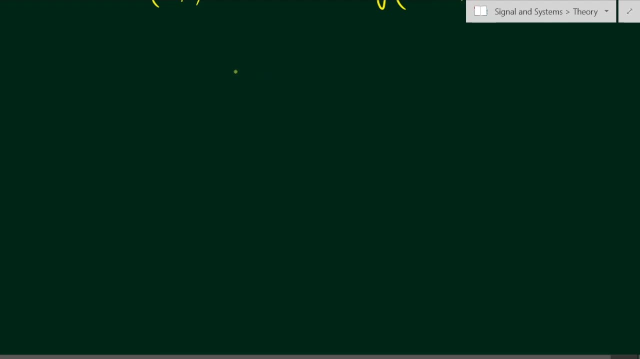 to the combined input signal response. So let me explain this. suppose this is a system with transfer function capital T. okay, suppose we give some input X of T and we have some output Y of T. okay, this output is the transfer function multiplied with the input. so suppose now we give two. 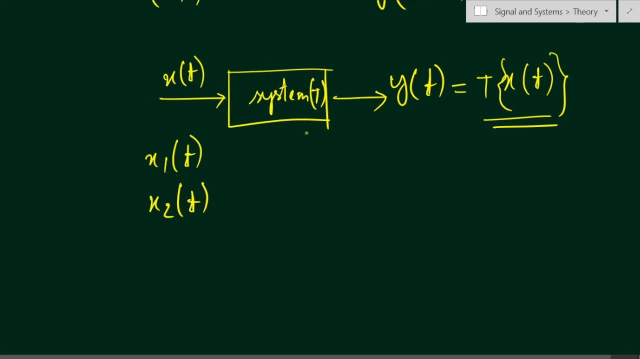 different inputs: X 1 of T and X 2 of T. so what will be the output? so suppose for this input, X 1 of T, the output is Y 1 of T, so this will be equal to T multiplied with X 1 of T, because this is the system response: T for the second. 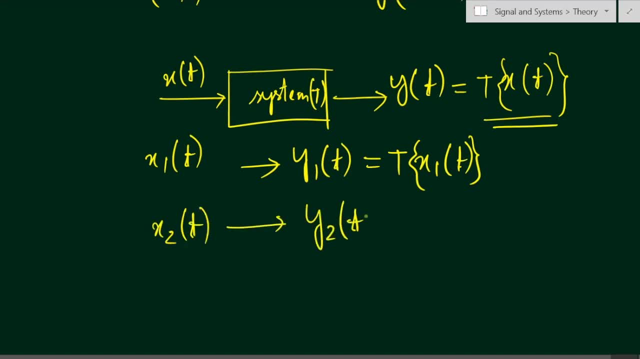 input. suppose we have, the output is Y 2 of T. okay, so what will be the Y 2 of T? T multiplied with X 2 of. so this will be T, X, 2 of T. now for this system. if we give this X 1 of T as the input, it produces Y 1 of T as the output. okay, and at the second, 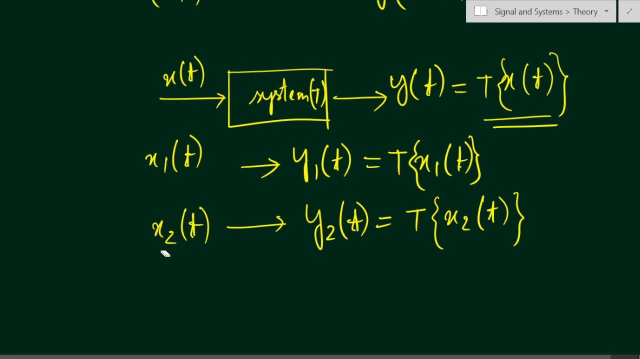 time. suppose, separately, we have given this input and we have given another input, X 2 of T, to the system and it produces some output, Y 2 of T. that is denoted by this. now we have to see if we give both this input signal at the same. 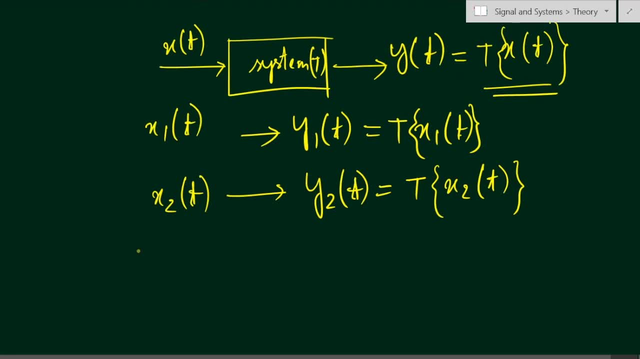 time to the system. so what will be the output response? so what will have Y equal to T of T inputs are given at the same time: X 1 of T plus X 2 of T. okay, so this is the transfer function, capital T. so these two input signals are given at the same time. 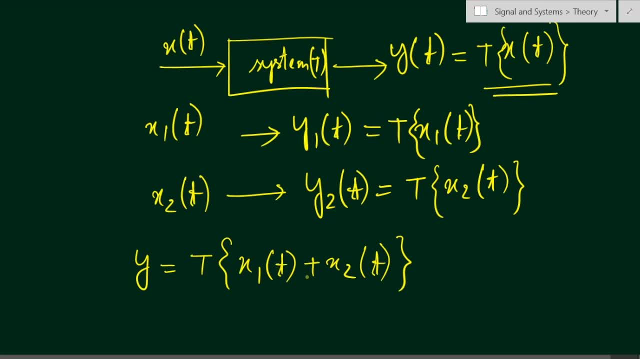 so what will be the output? so this is the output. so if this is equal to Y 1 of T plus Y 2 of T, then this is called as the additivity property. if this combined input signals produces similar kind of output, that is the combined output. y is equal to the individual sum of: 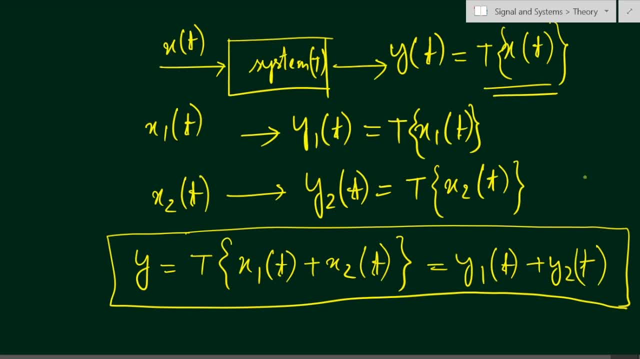 output, then this is called as the additivity property. First of all, we have seen this is additivity property. That means for a system to be linear system it has to follow two conditions. One is the additivity property. So we have seen this is the additivity property. 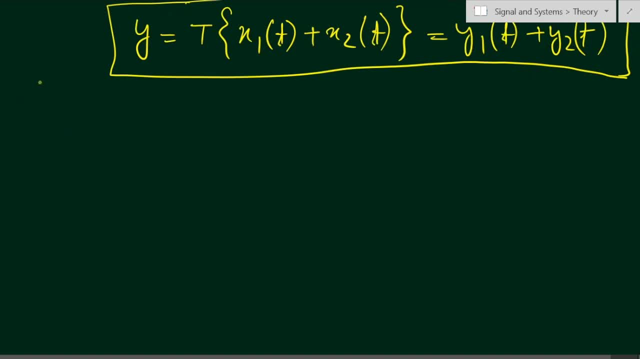 And the second condition is it is it has to follow the homogeneity property. The second condition for a linear system is homogeneity, Or we can say that it is scaling, scaling property. So what is the scaling property or what is the homogeneity? 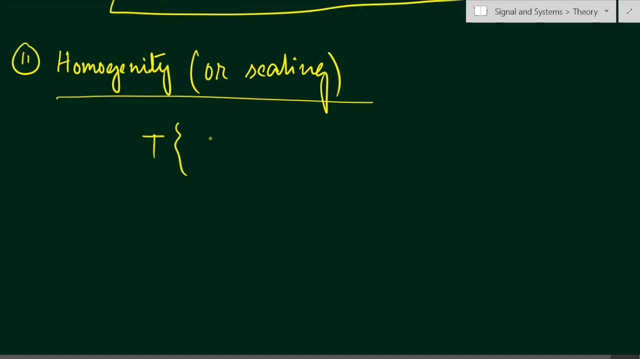 The transfer function multiplied with some time scaling, factor AX, So it will produce AY. So if it produce the same amount of time scaling, so this is the scalar quantity, This A is the scalar quantity. A is nothing but a scalar quantity here. 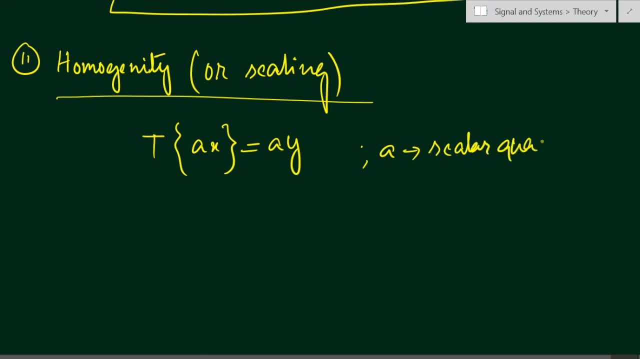 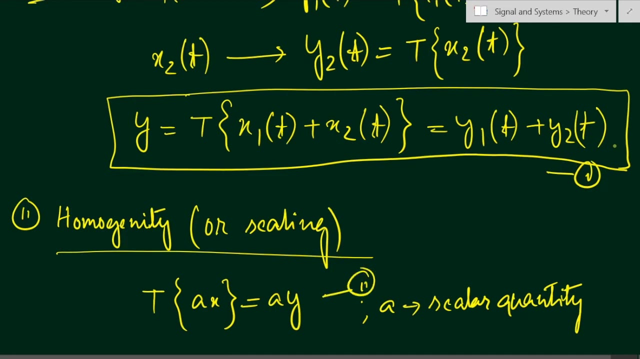 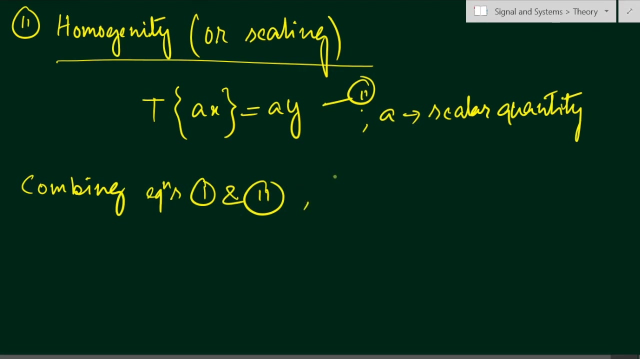 A is a scalar quantity. If we get the same scaling at the output, then it is called as the homogeneity property. Suppose this is number one and this is number two. equation Now combining equations one and two. So, combining equations one and two, what we'll have? 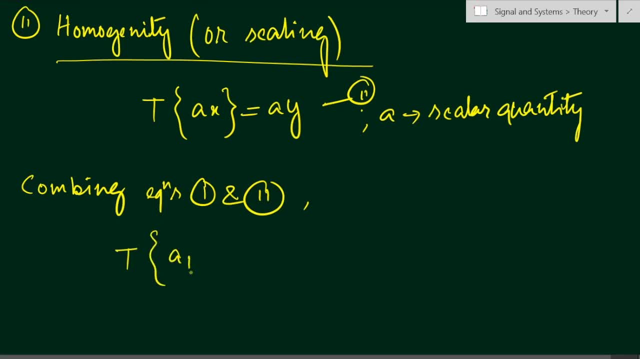 We'll have here T of, suppose A1X1 of T plus A2X2 of T. We have applied the additivity as well as scaling property at the same time. This would be equal to A1Y1 plus A2Y2.. 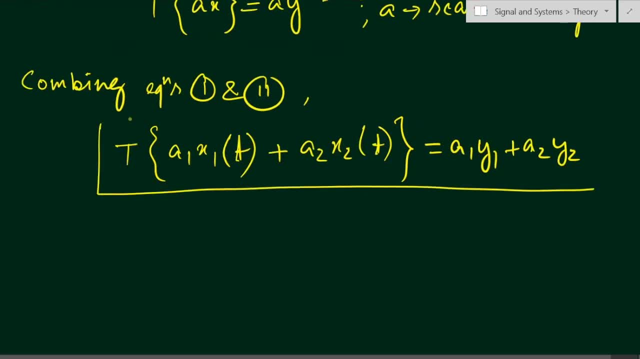 So you have got this. So this is as a whole. This is called as the linearity property, or we can say that this is the superposition property. So here, A1 and A2, these two are the arbitrary scalar quantity. So for the time invariance property we have already seen in our previous lectures. please, 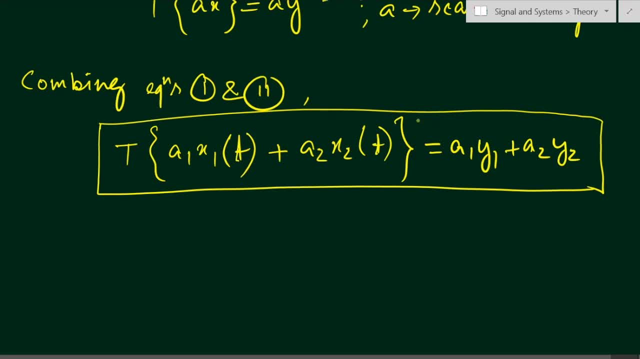 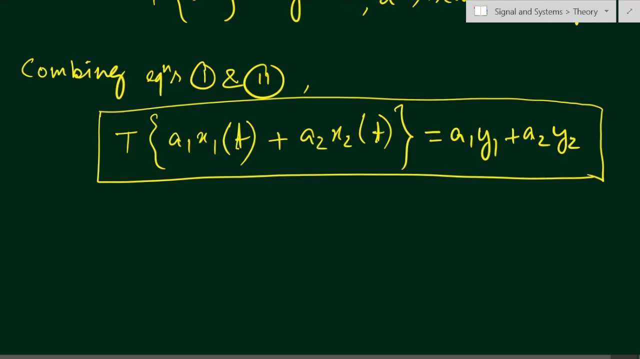 go through it Okay. So in the case of time invariance, we have seen that time shift- okay- at input produces or causes same time shift at the output. Now let me explain this with some examples. So let me take one example. 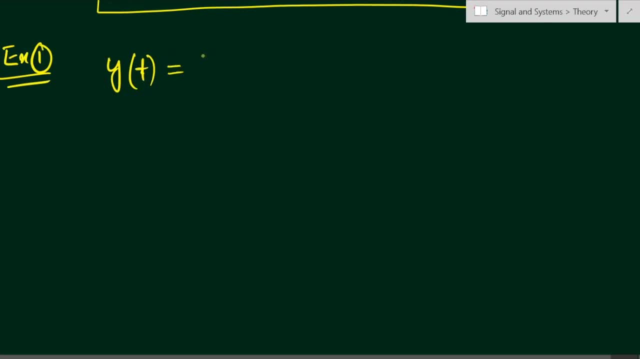 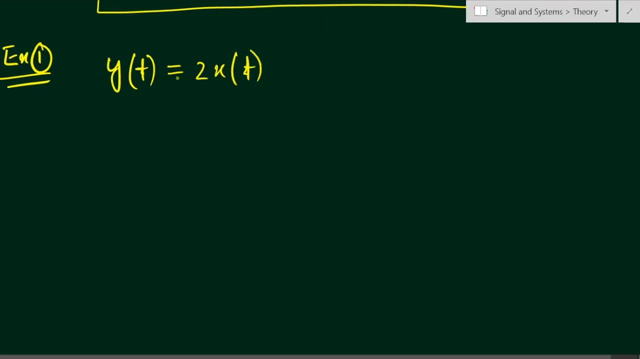 We have a system: output denoted by Y of T is equal to two X of T. So this is the first example. Suppose we have the input output relationship is this: one: Y of T is equal to two X of T. Now for input X1 of T, what will be the output? 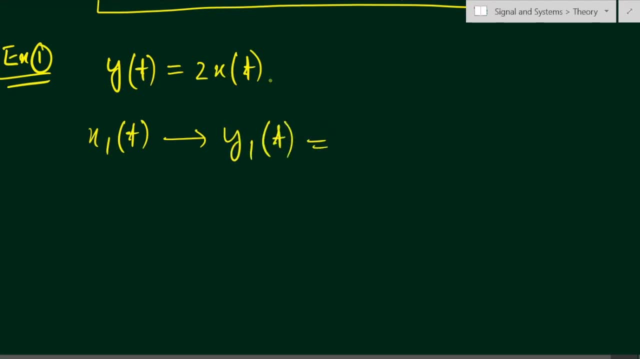 Suppose the output is Y1 of T, So this will be equal to using this equation, two X1 of T. If we have another input, X2 of T, So what will have? the output is suppose Y2 of T, So what we'll have? 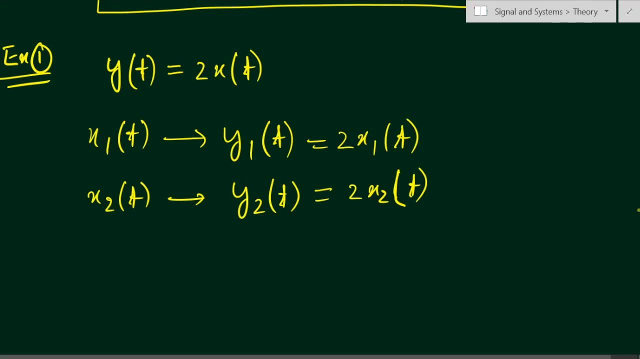 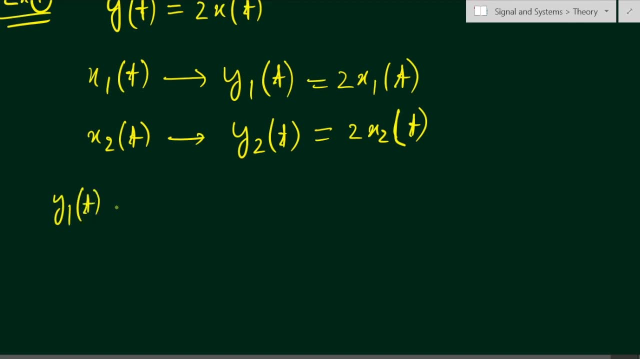 Two X2 of T of t. Now if we add these two outputs, that is y1 and y2.. So what will happen? y1 of t plus y2 of t is equal to. so what will have? 2x1 of t plus 2x2 of t. So this we can write as 2 if we take 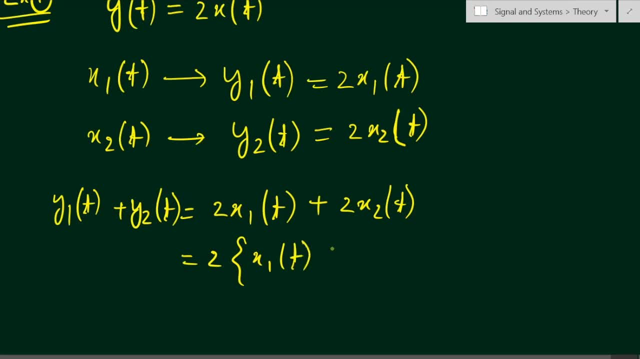 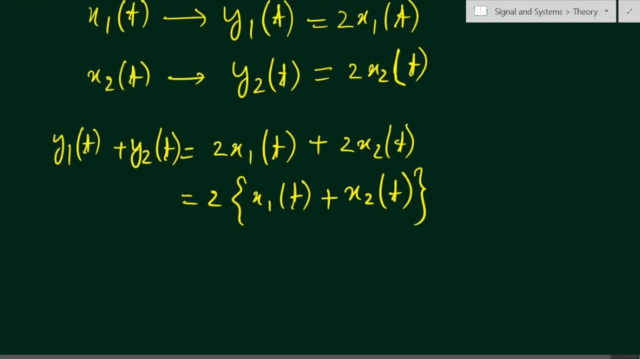 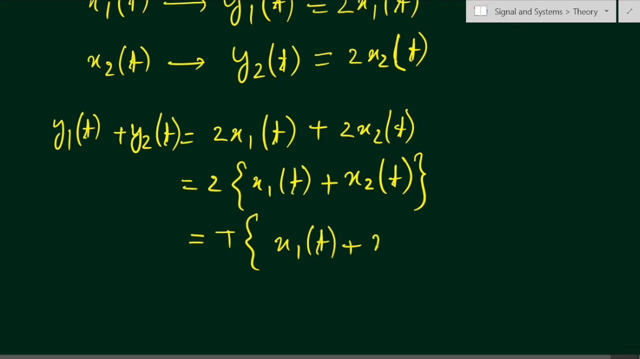 common what will have: x1 of t plus x2 of t. This two is nothing. but this is the transfer function here, because we have the input is y of t and input is x of t. So we can say that, so we can write it as t whole into x1 of t plus x2 of t. So this given system has followed the linearity. 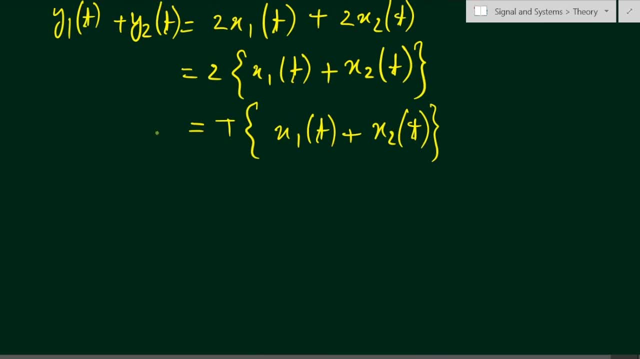 properties. So this is called as the linear system. Therefore the system is linear. So for linear time invariant system, we have to check whether the system is linear as well as we have to check whether the system is time invariant. Now we will check the time invariance property For time invariance. 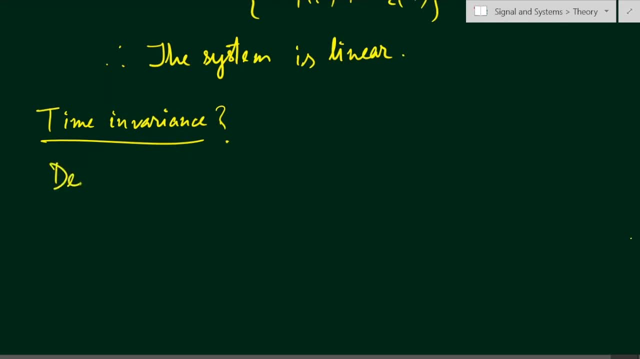 property we have to put some delay in input. Therefore delay in input by t naught. So we have assumed that delay in input. we have t naught delay and let the output be y1 of t. This y1 of t will be equal to 2 into x1 of. 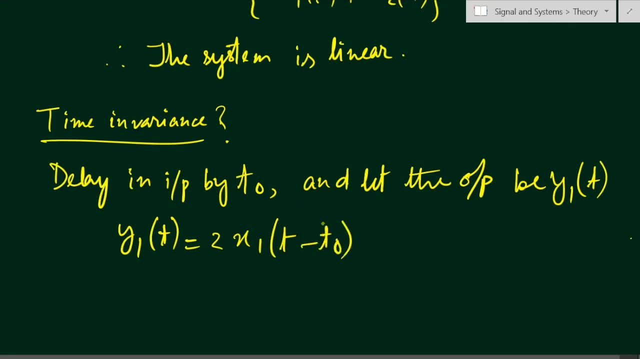 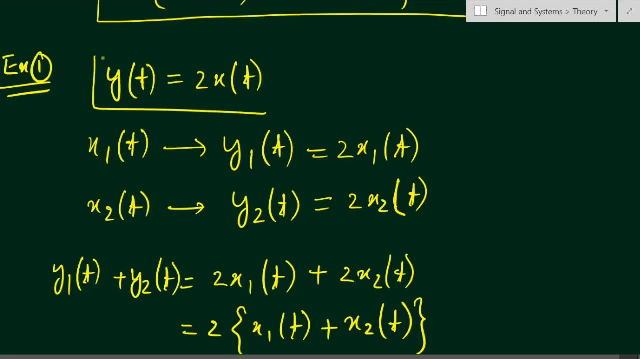 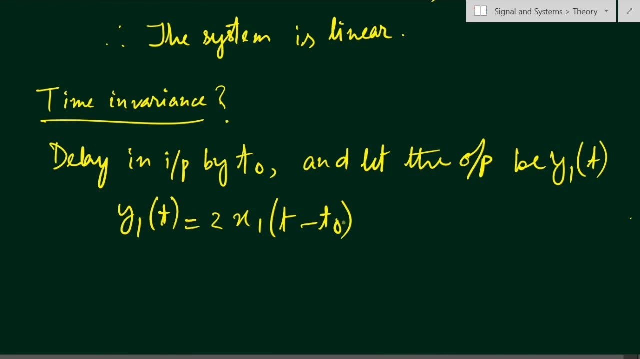 t, t minus t, not, because this is the given input delay. that is, now. the input signal becomes this: t minus t, not. this one is a given equation. Okay, so using this given equation, we have found out the output. So we have got this output for the input delay. Now we have to put some delay in output Now. 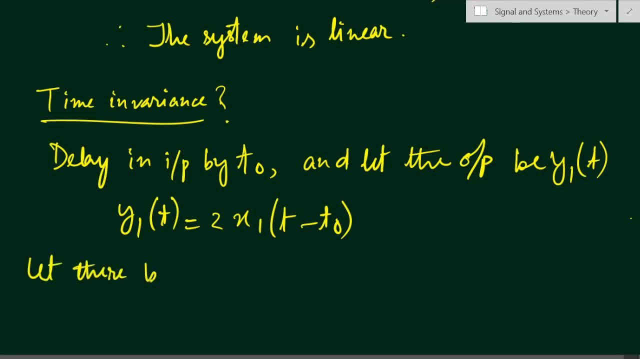 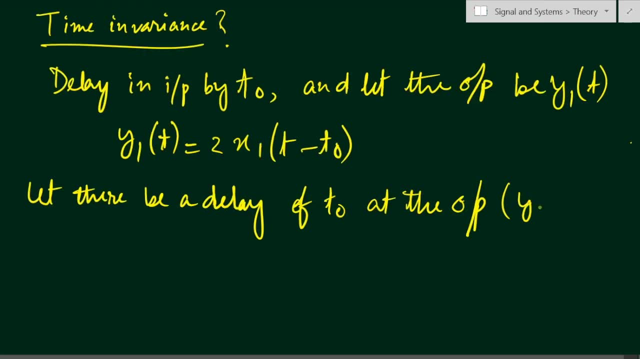 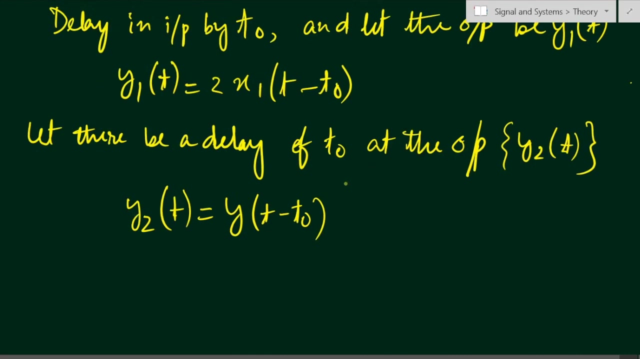 let there be a delay of t, not at the output, and the output is suppose y2 of t. So what will happen? y2 of t is equal to y of t minus t, not because we have put some delay in output. So using the 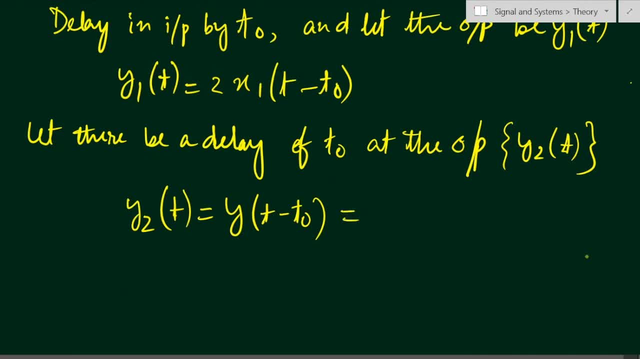 given equation, what will have? we have to replace t with t minus t, not. So, using this equation, we have to replace this t with t minus t naught. So we'll have 2x of t minus t naught. So here, in this first case, we have applied some delay in the input. 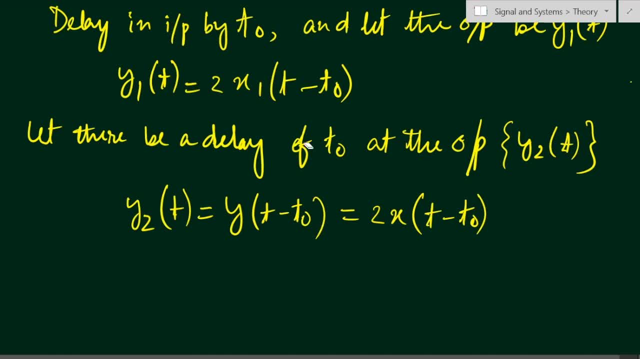 In the second case we have applied some delay in the output. Okay, same amount of delay, So what? we'll have these two right hand sides, so this one is equal to this much. So we have seen that y1 of t is equal to y2 of t. 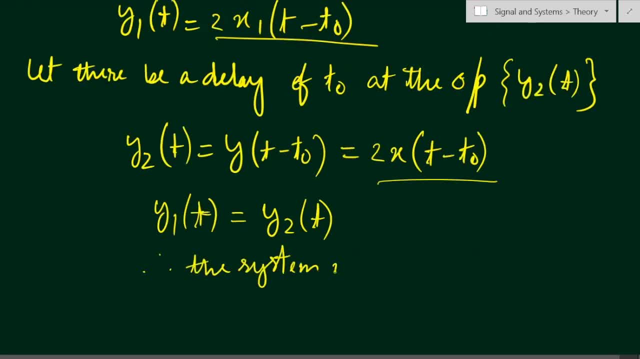 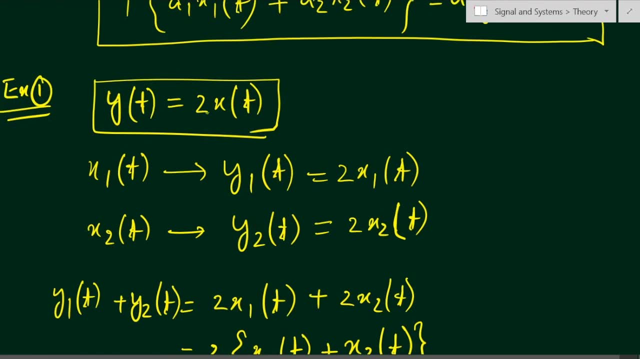 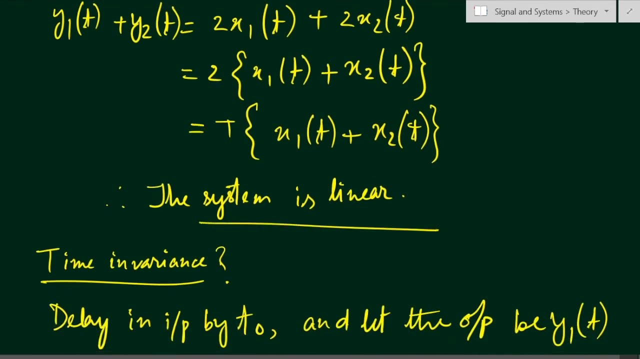 Therefore, the system is time invariant. So for this given system, denoted by y of t, is equal to 2x of t. This system follows linearity property, that is, the system is linear as well as it is time invariant. Therefore, we can say that the system 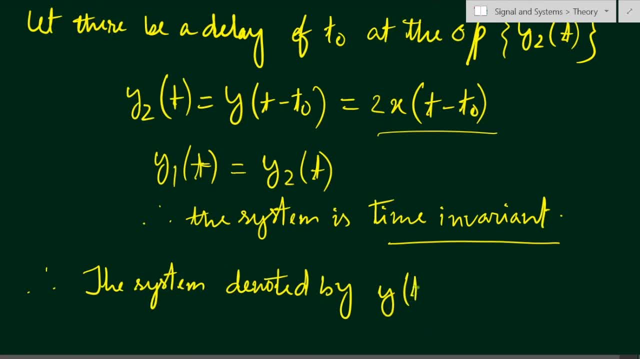 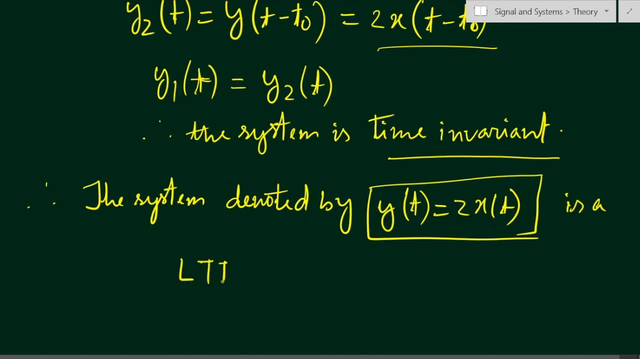 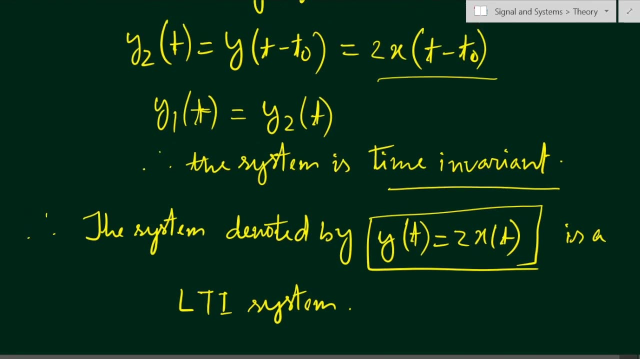 Denoted by y of t is equal to 2x of t is a LTI system or linear time invariant system. So in this lecture we have seen what is a linear time invariant system. So, in brief, we have to keep in mind that a system is said to be linear time invariant.